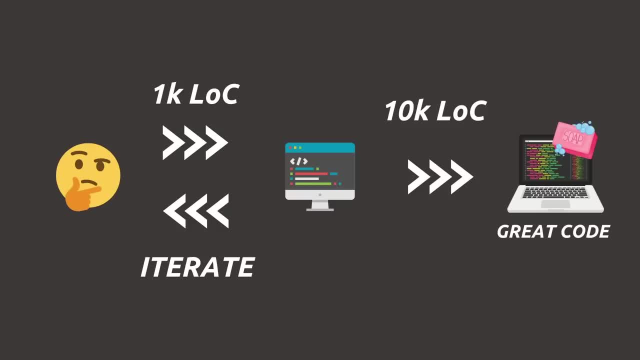 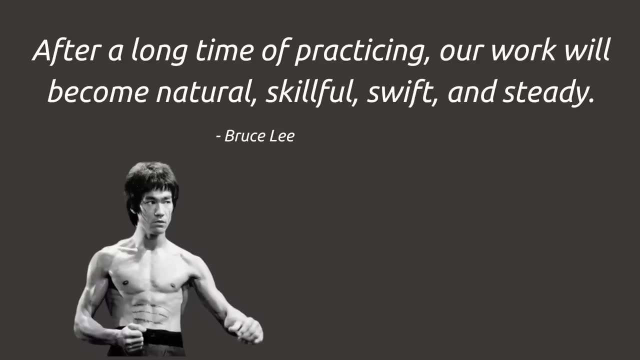 lines of code where every thousandth line is better than the last one. Coding or programming is a craft and you get better at it when you're doing it, So I'm going to show you how to do it By being inefficient, slow and bad. it's a lot more like woodworking playing an instrument. 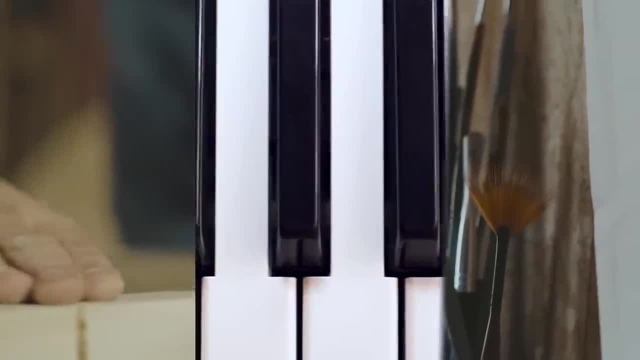 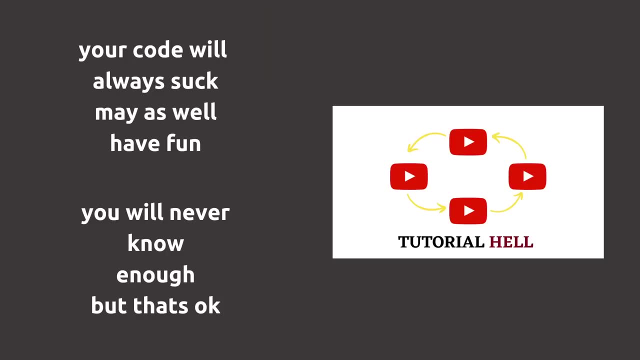 drawing than it is like law or history or finance or anything that's very information dense. Finally, this point, or this mindset, is really helpful in making you avoid tutorial hell, And if this video reaches, say, 10 likes, I'll make a step-by-step guide on how to get out of. 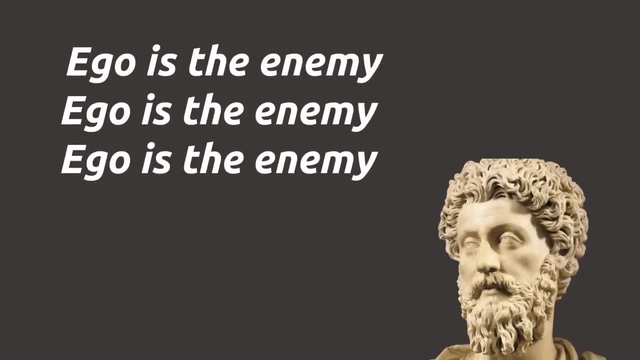 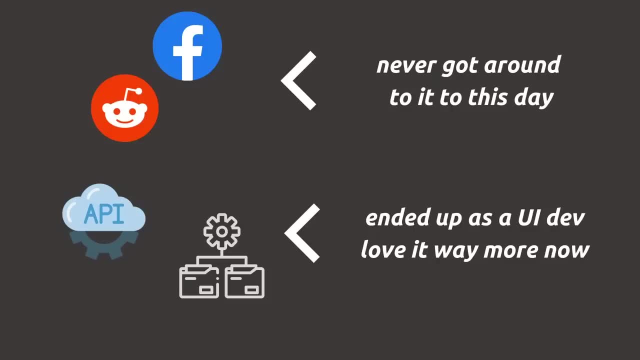 tutorial- hell, All right. point number two is: ego is the endgame. So when I was just getting started, I didn't want to do the plain HTML CSS recipe websites that tutorials get you to make. I wanted to do the cool stuff. I wanted to make my Facebook clone. 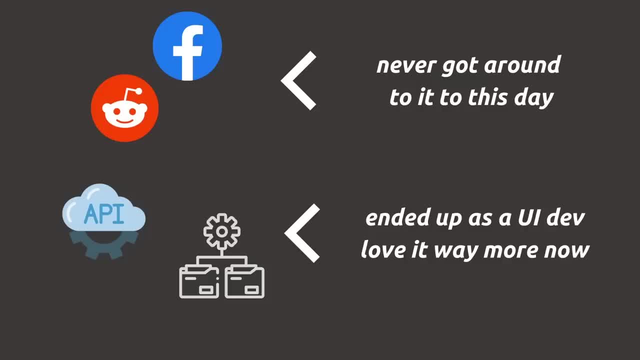 or a Reddit clone. I wanted to be nitty-gritty in algorithms and REST APIs. This was my ego speaking. Had I swallowed my pride and not thought that doing these basic things were beneath me, I would have become a much better engineer in a lot. 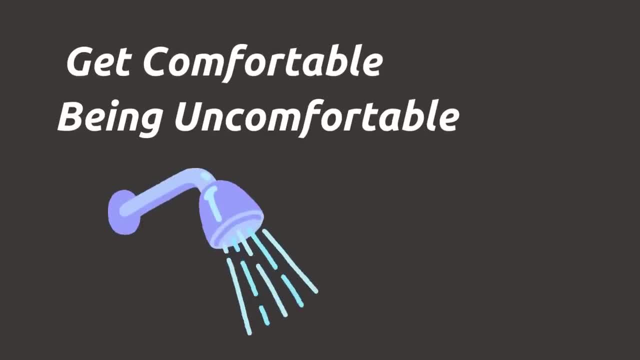 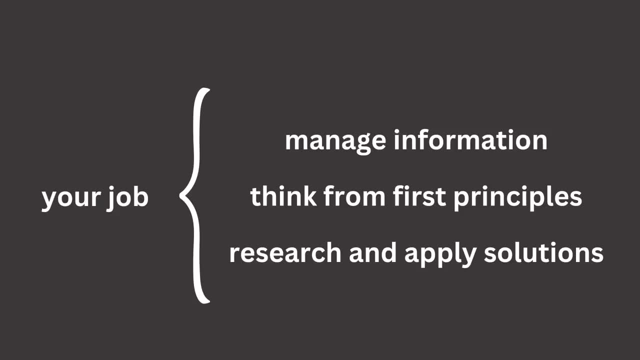 less a time, All right. so point number three: get comfortable with being uncomfortable In software engineering. you're an information manager, So it isn't your job to know everything, And as a professional developer, you'll never know everything. However, given that the problem 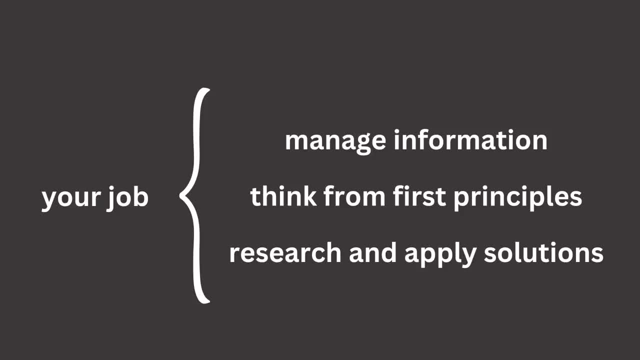 is within your domain. so say, you're a backend engineer and it's a backend problem, you're expected to be able to go and solve it, And that's a really uncomfortable feeling And it's going to be very uncomfortable. I mean, tools will be there and you can read up as much as you. 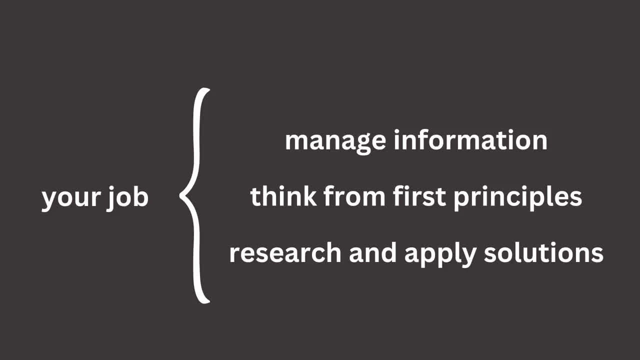 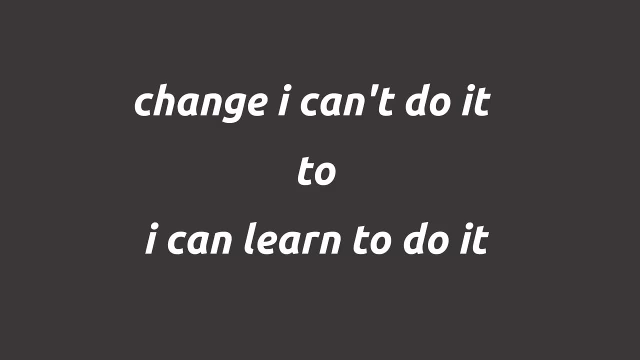 want outside of work. but there's so much in this field that you just have to be okay with feeling uncomfortable And you have to sort of learn to enjoy it. You have to see it as a part of the job that you actually enjoyed, Like, okay, cool, I'm not uncomfortable, I'm actually going. 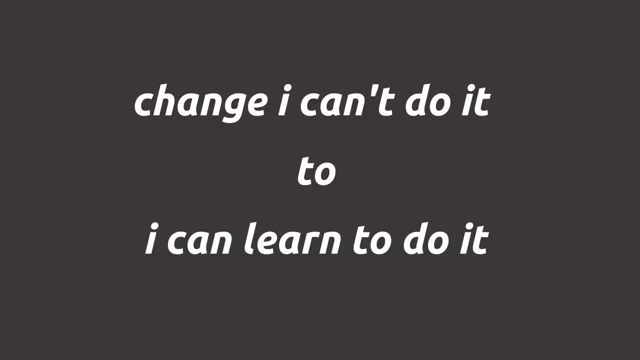 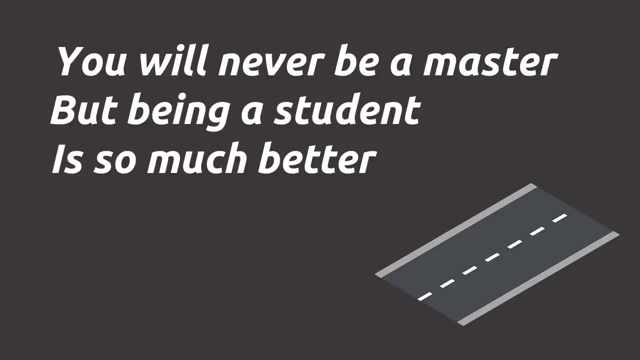 to learn something. now I'm going to go beyond what I knew before I picked up this piece of work, And that's the beauty of this field. So the final point is: you will never master programming. I see these kind of posts on Reddit all the time. How quickly can I master X language? Or is it better?